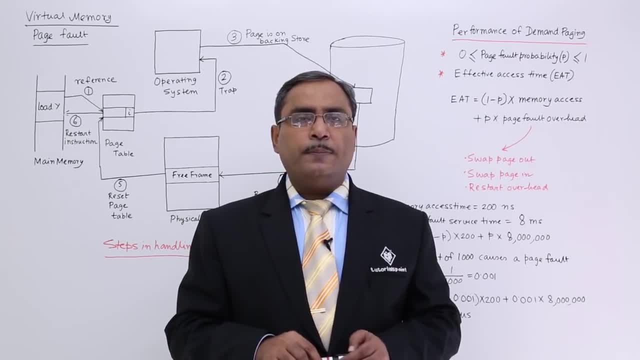 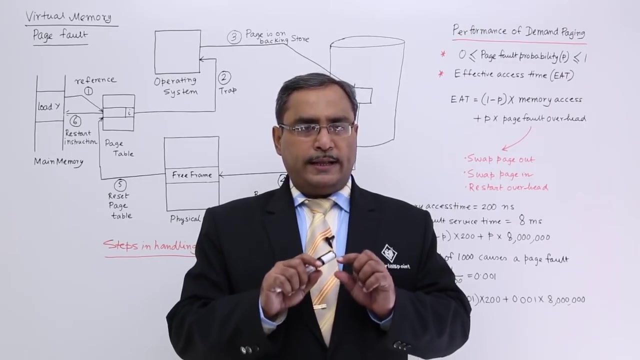 Point number 3, the page is not available in the main memory. Who will tell that one The same page map table? because in case of virtual memory, we have seen that. in case of virtual memory, we have seen that each and every row in the page map table is consisting: 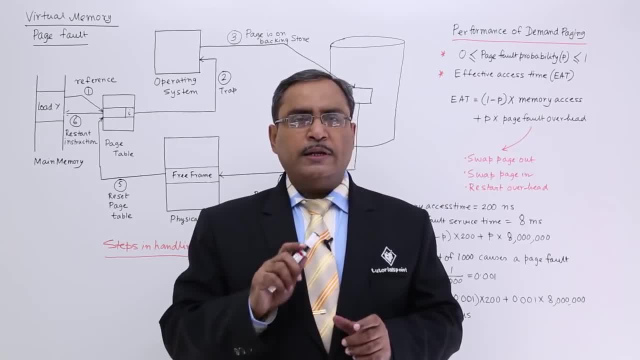 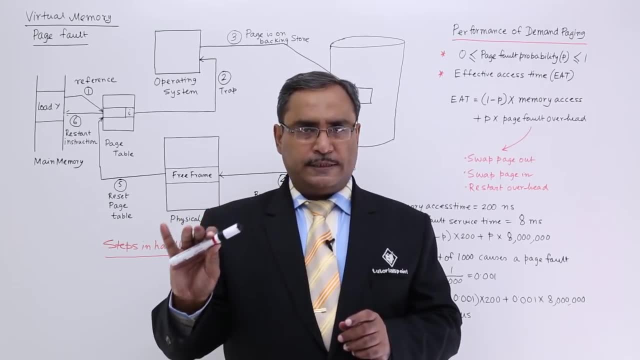 of two fields. One is the frame number and another one is the valid invalid bit. Valid bit means this page is existing in the main memory, So the page is not available in the physical memory. against the frame number, as mentioned in the other field. But if the 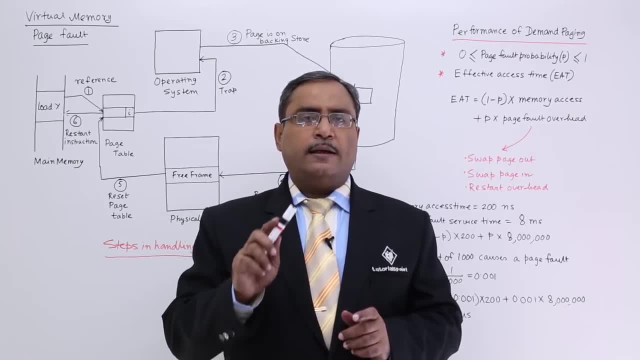 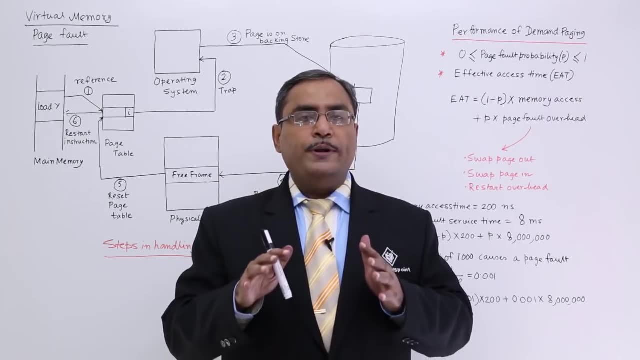 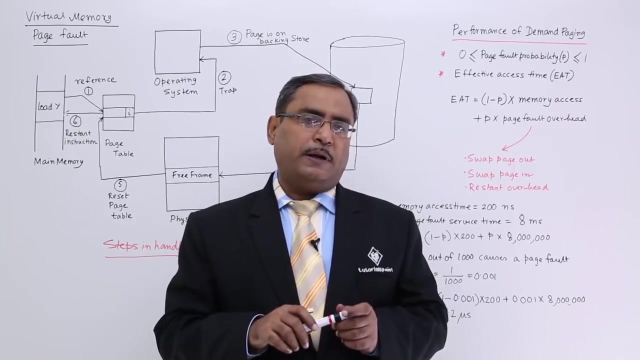 valid- invalid bit is invalid. that indicates that the page is not existing in the main memory. Then the situation does arise, will be known as page fault. So how to handle the page fault, that will be discussed in this particular topic, in this particular session. 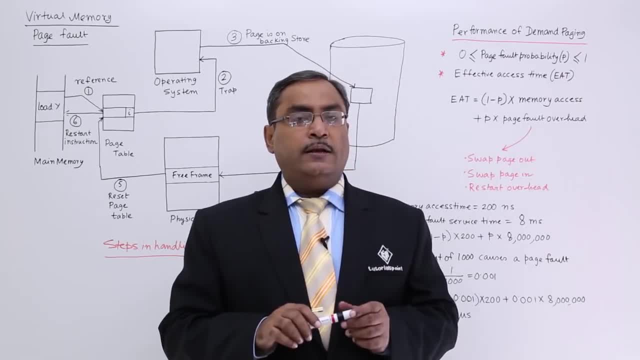 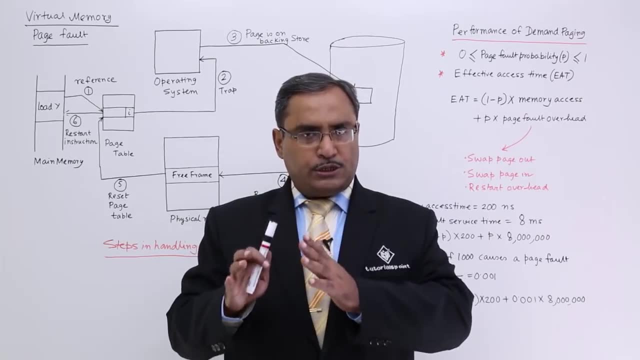 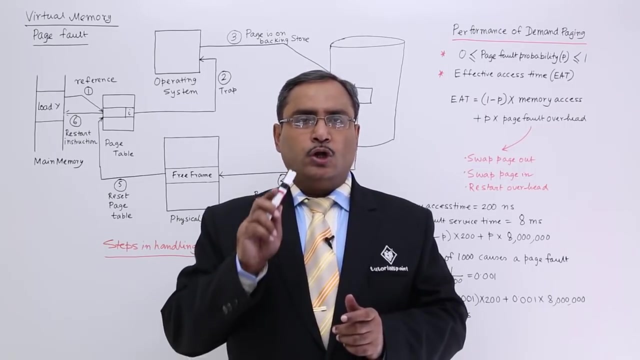 So now, whenever a page fault will take place, Then we shall have to search the required page onto the secondary storage. After getting the required page content on the secondary storage, then we shall have to find a free frame. While finding free frame, two things can take place. Point number 1, free frames. 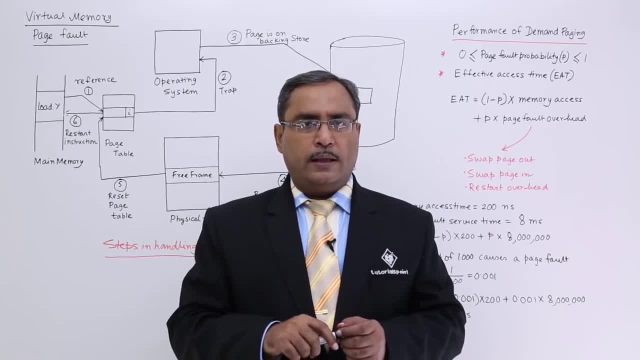 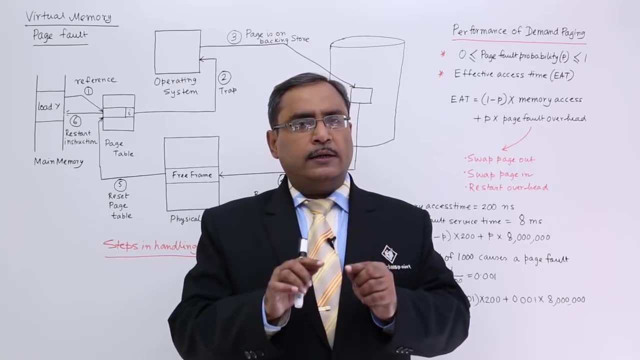 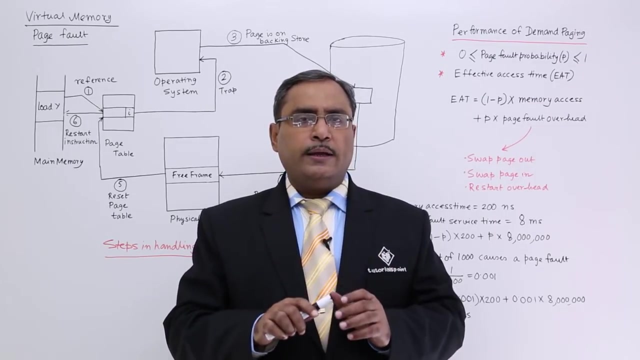 are available, So the new page will be brought in there. Point number 2, the free frame, is not available, So I shall have to replace some other previously loaded page to make a room for the new page to be brought in. So in this way, this particular 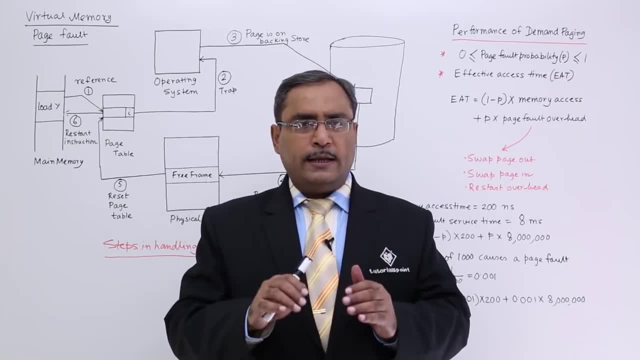 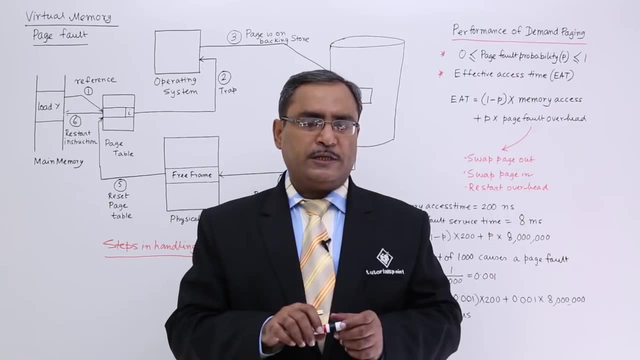 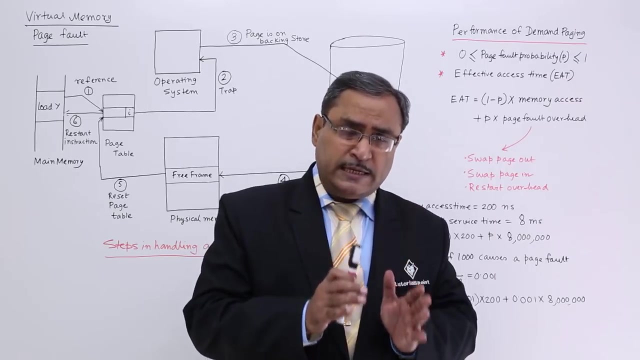 page fault will be handled Whenever we are getting a new frame. where we are getting a new frame available, there is no need to have any kind of page replacement algorithm. But whenever we are loading a page to a frame replacing some previously loaded pages, then 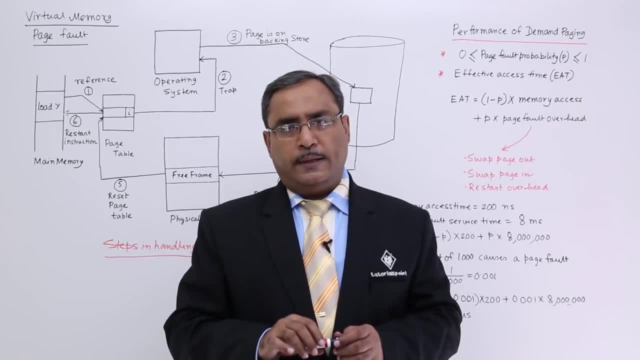 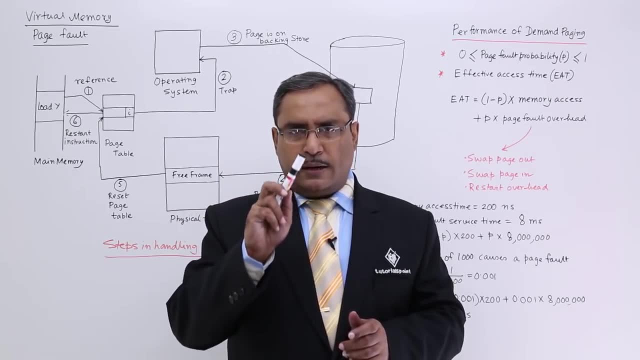 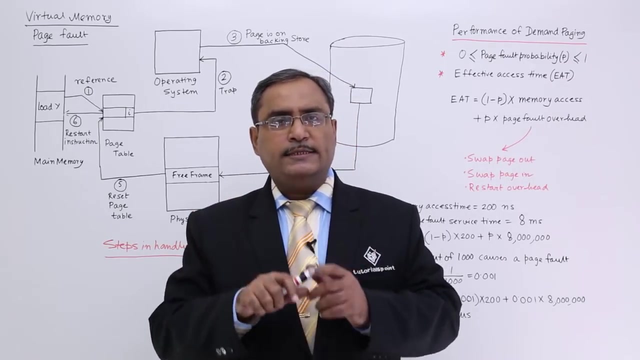 the page replacement algorithm will come into the play And whenever the corresponding page will get loaded to one of the frames, then again the particular page in the page map table, the invalid bit, will be made valid, because now it is physically existing onto the physical memory or main memory. 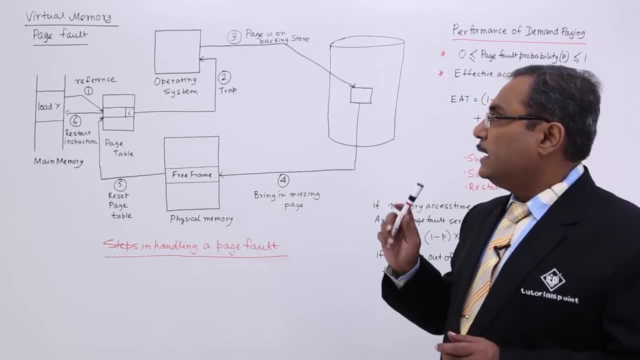 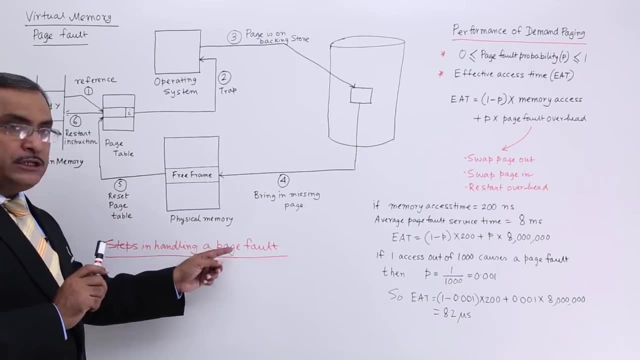 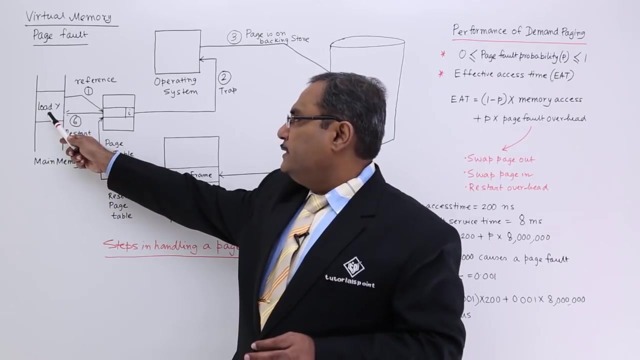 So let me go through this diagram. This diagram will depict all these details. Okay, now see, here we are having steps in handling a page fault- suppose this is my main memory. here the program is executing and in this particular program there is a particular page which is now having its execution. let us suppose there is one. 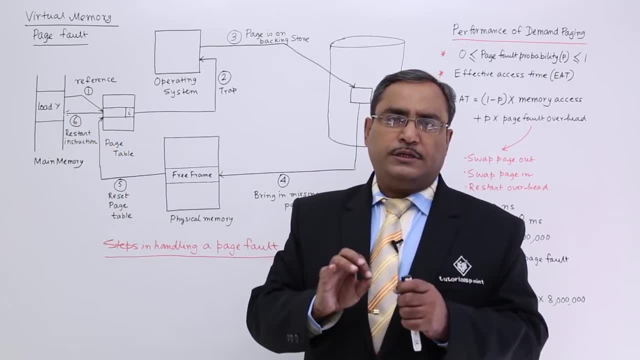 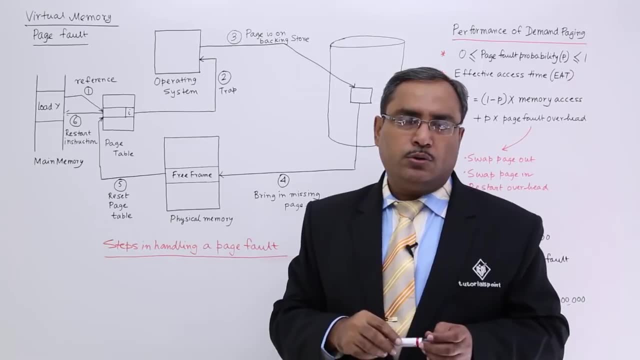 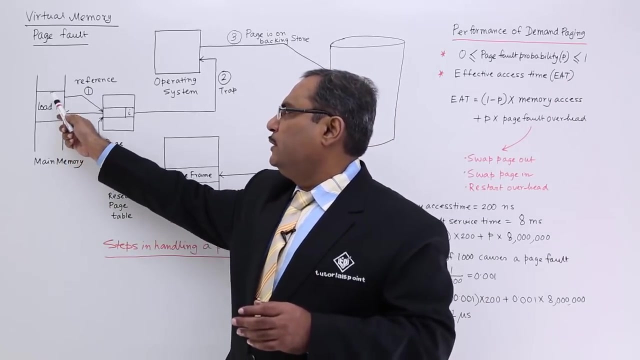 instruction that is load y. so one instruction is there that is load y. but this load y is not available in this particular page. so it is asking for a new page, say, say y be the a new page number, so load y. so this particular page is not will will not get the control. 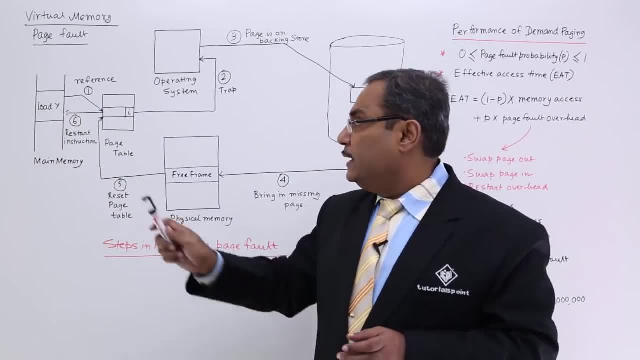 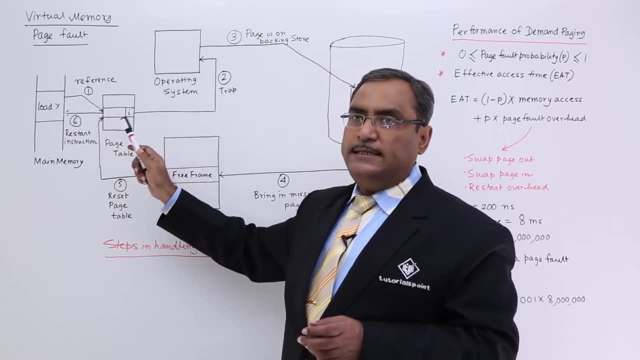 the control will be transferred to the page number y say so. now. it will be mapped onto the page map table and it will check whether this particular page is existing in the main memory or not. but at this particular reference we are getting that the page is not available. 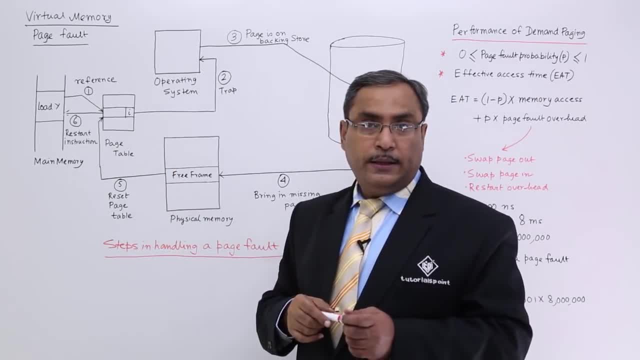 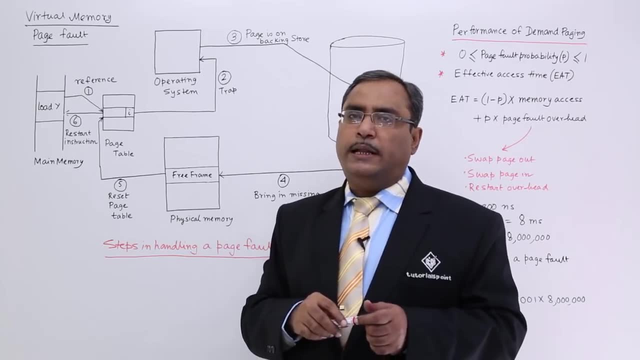 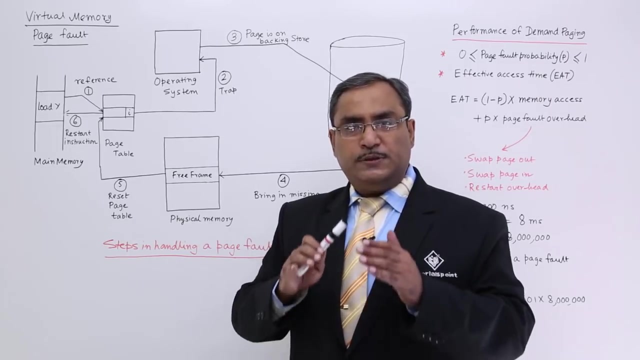 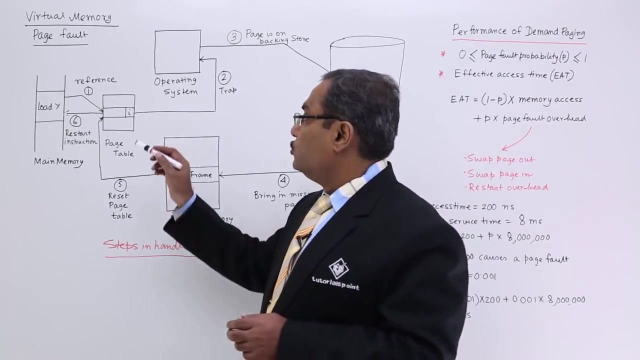 in the main memory. so the bit is invalid. so this particular thing will produce trap. trap means highest priority. non maskable interrupt. that means it cannot be masked, that means it cannot be ignored. that means operating system is bound to pay attention to this particular source of this trap, addressing error. so now it will go to this particular operating system. 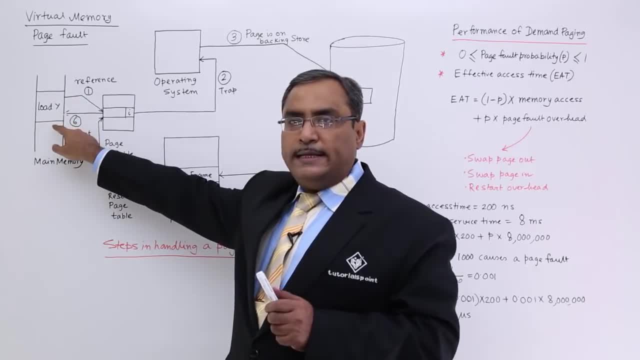 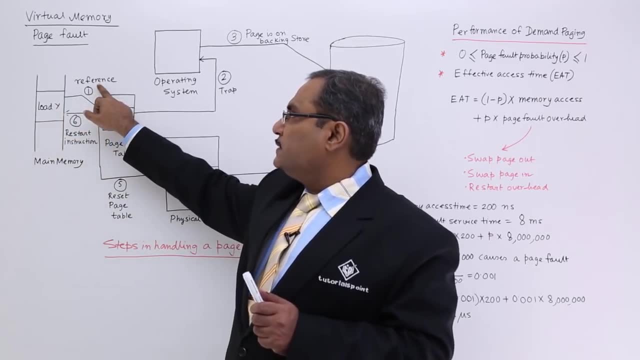 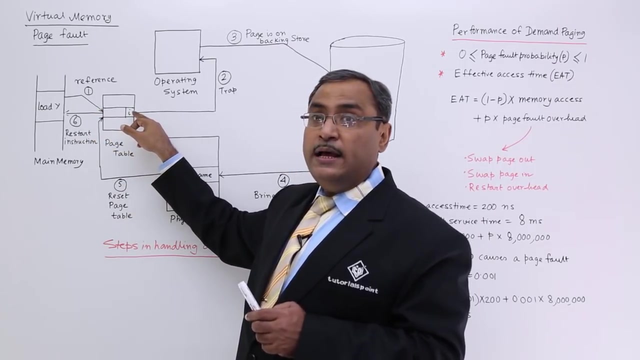 so what is the step one? there is a particular page which is now in execution. there, one page has been requested which is not in the memory, so how can i get that one? at first, the reference will be searched onto the page map table here. against this particular page, i am getting the value i. i stands for invalid means, the 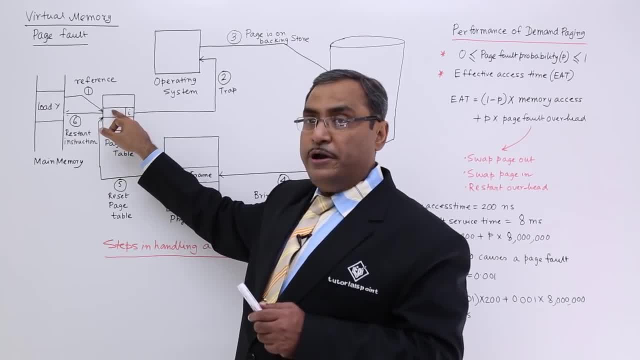 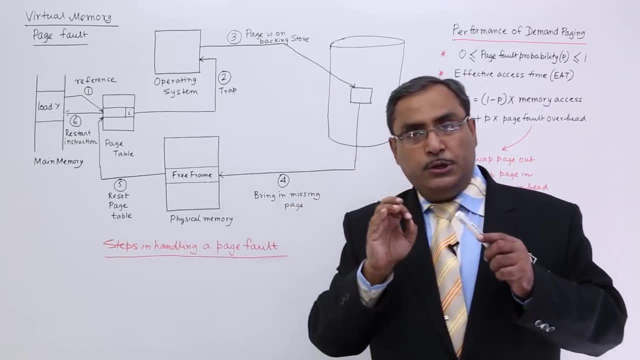 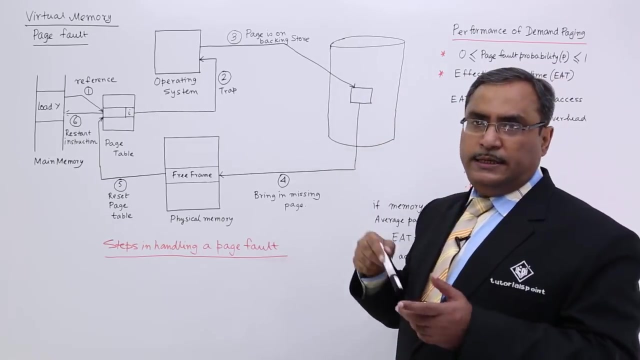 page is not available, so there is no valid frame number written here. so it will be indicated as a trap to the operating system. now it is the purpose or the duty of the operating system to search that particular page onto the secondary storage. so this is a drum, that is a disk. so 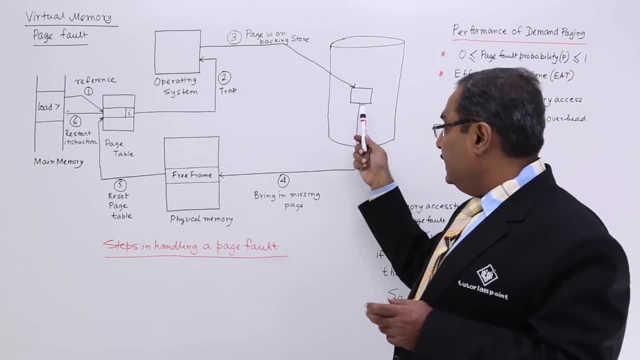 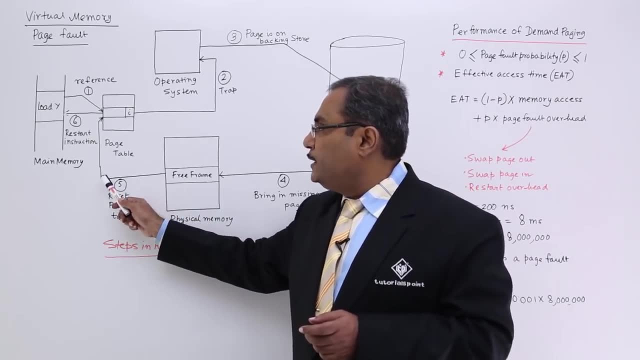 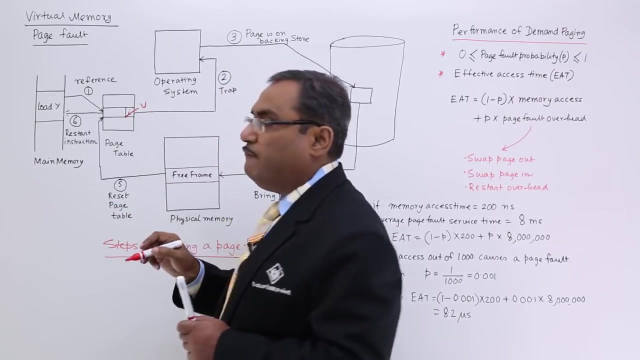 on the secondary storage, the page has been found and then the page will be brought onto a free frame. this free frame, the frame number, will be written to this particular location and obviously this particular i will be replaced by v. v stands for valid. let us suppose here: 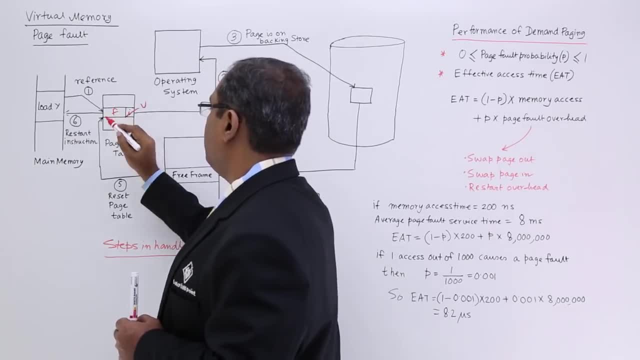 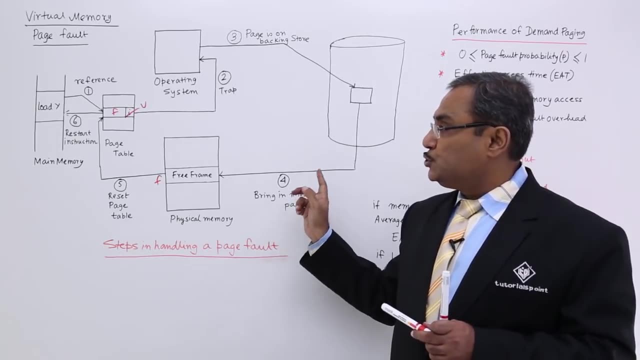 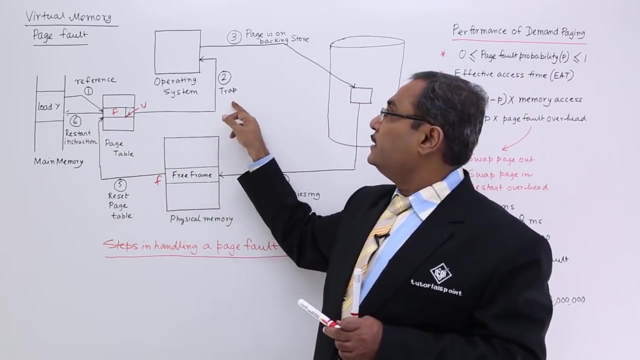 the frame is f, so here f will be written. so in this way the page fault will be handled. so in this diagram we have shown that. what are the different steps? so step number one: reference. step number two: trap addressing error. step number three: page is on the backing store. 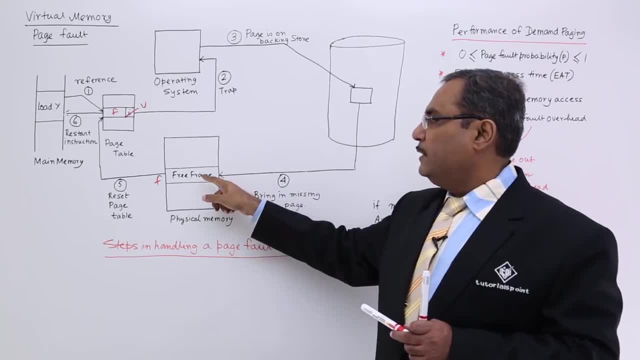 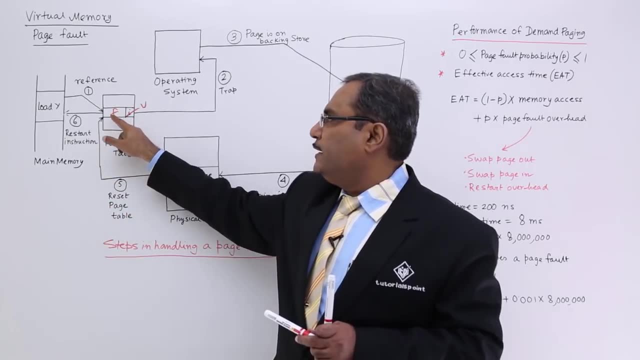 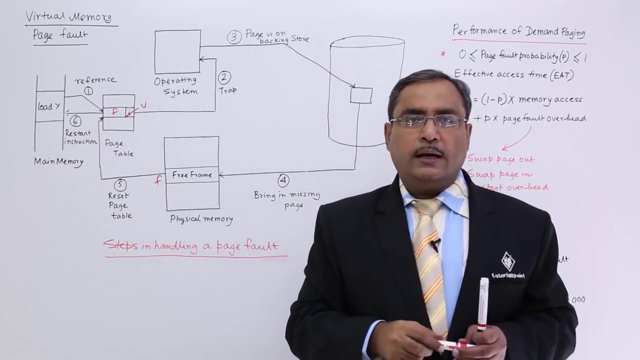 page number four: bring in the missing page onto the free frame. page number five. step number five: restrict page map table. so reset page map table means f will be written here and step number six: restart the instruction, because already the page is now in the main memory. so page number six is the value of the page. so we arrive at a page. value of the page. 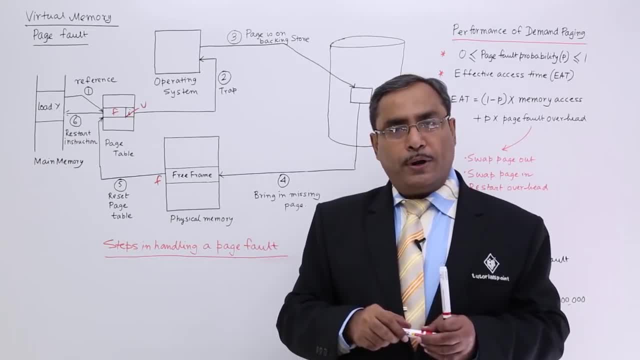 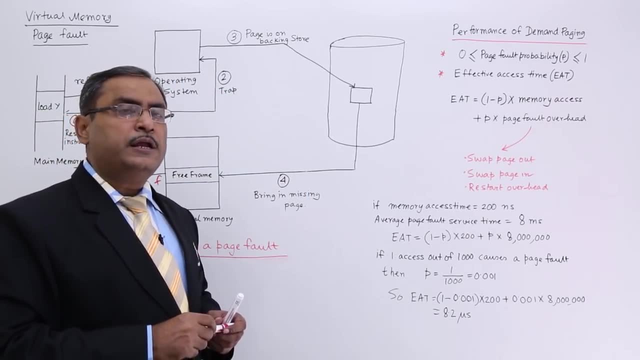 so this is the definition of a page fold. so in this way the thing will take place. i think you have got this, a particular idea, the how a page fault can be handled by the operating system. so now here we are having one formula. it is a very famous formula, different numerical. 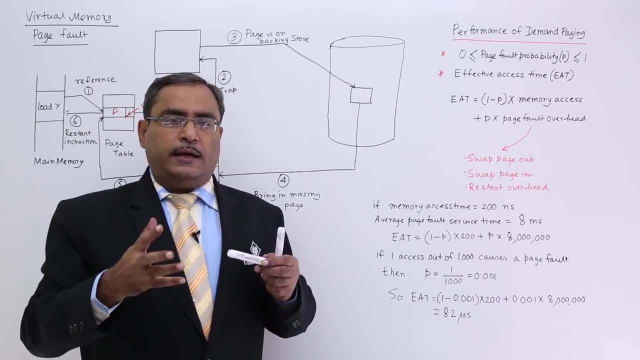 problems will be coming based on this particular formula. we know that page fold probability that means if i, if i, if i, ahem, ahem, ahem, if i refer 1000 pages, then how many times the page will be fetched? we have to think about it and this is the key thing that we should. 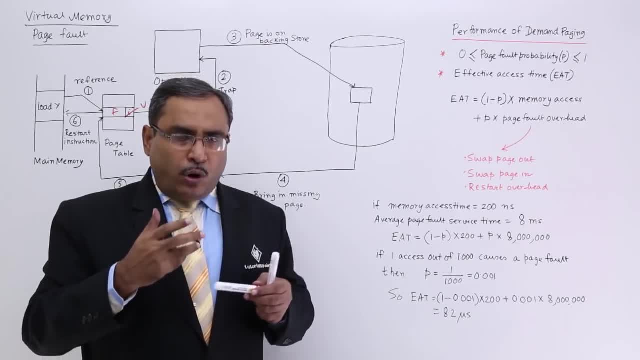 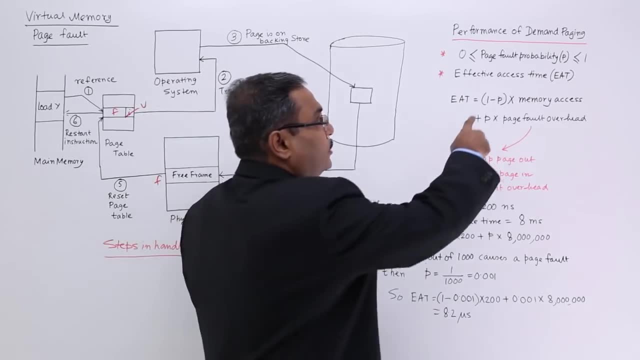 times the page fault may take place. So if you go on calculating in this way, so now whatever the figure we are getting is known as the page fault probability. So we know that each and every probability can be ranging in between 0 to 1.. So that is a probability. 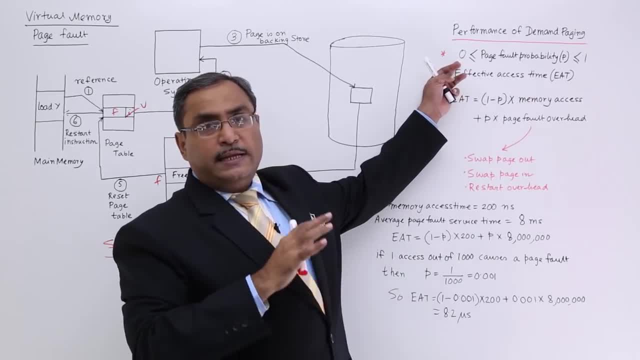 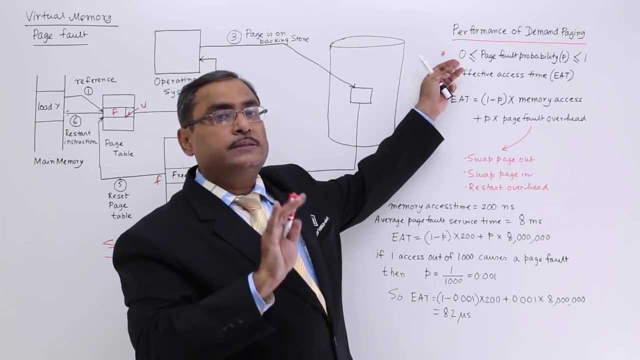 value 0 means. what Means? that is no page fault? There is no probability of page fault. That means all the pages are already there in the main memory somehow. So that is why, whenever a page will be referred, it will be found in the main memory. But what about? 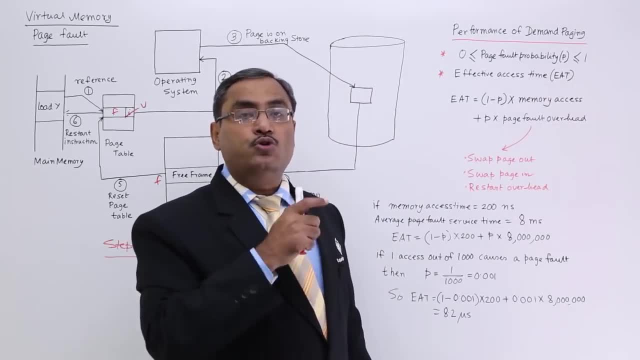 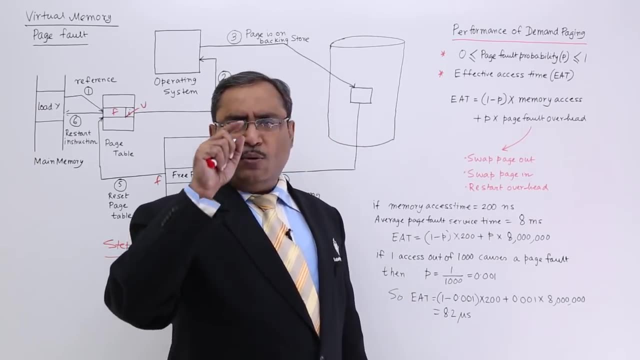 the page fault. probability 1? Means page fault is bound to occur. When, Let us suppose, there is a single frame on which a program or process is executing, Then what will happen Whenever a new page will be called? obviously the page would not be found in the main memory, So 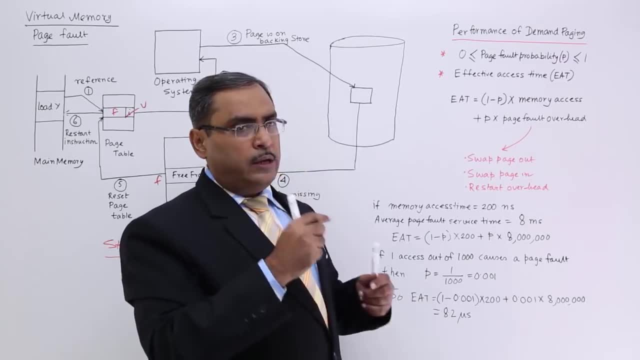 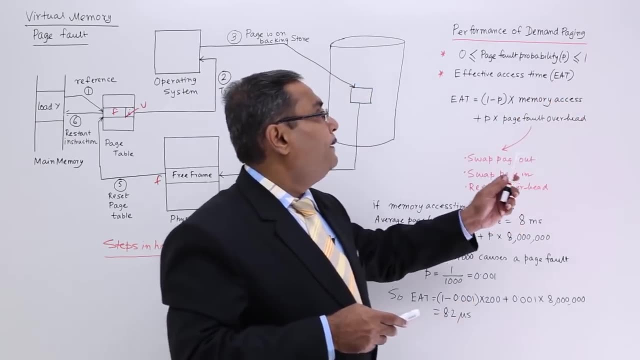 each and every time there will be one page fault. So whenever a new page will be referred, page fault is bound to occur. In that case the page fault probability will be 1.. So effective accessing time- EAT- can be measured in this way. What is P Page? 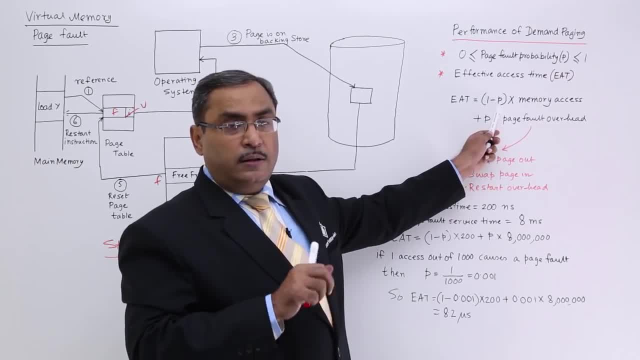 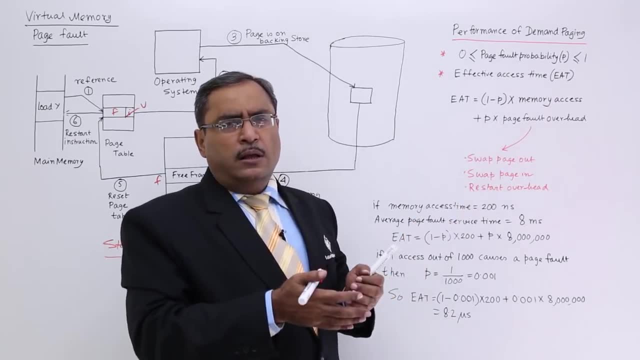 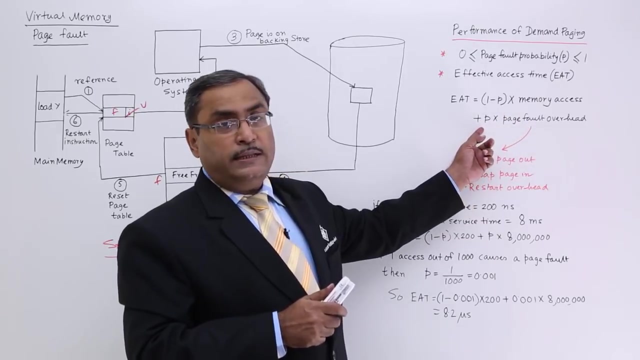 fault probability. So 1 minus P means probability of no occurrence of page fault. So that will be multiplied with the memory access time, because there is pages already there in the memory. So memory accessing time will be multiplied with it. What is P? That is a page. 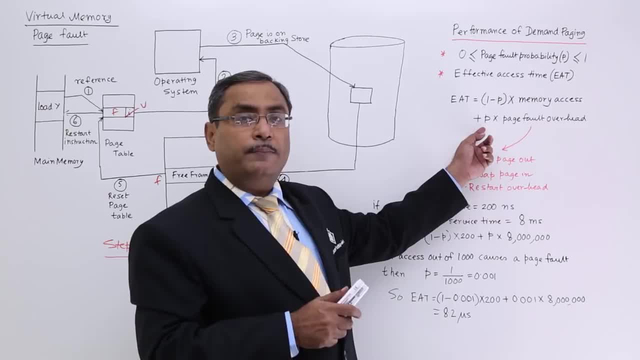 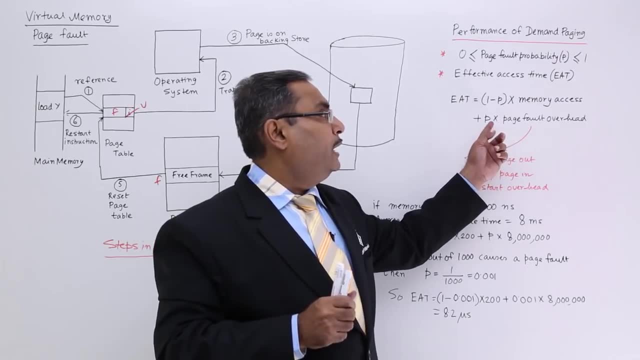 fault probability. So whenever this page fault probability will come, then this page fault handling. So to tackle this particular page fault situation the time required will be multiplied with that. So page fault overhead It is having mainly three components: One: 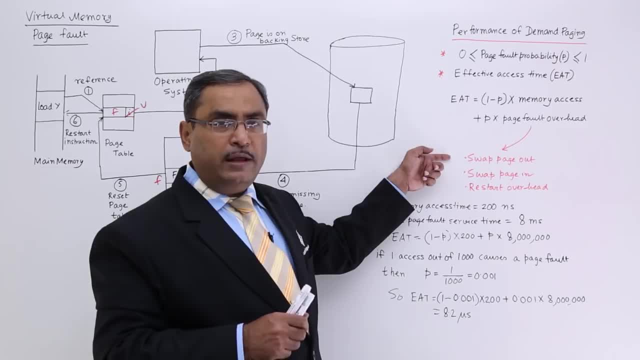 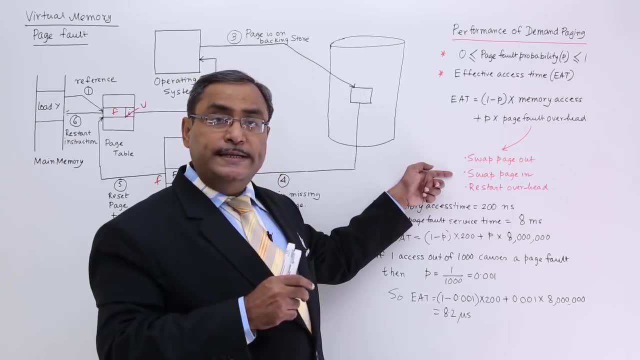 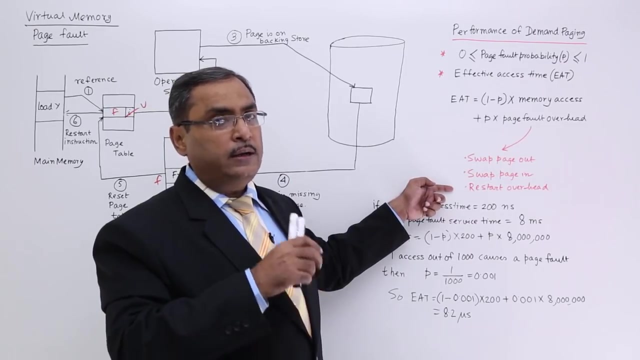 is the swap page out. If there is no free frame available, then I shall have to swap out some initially loaded pages and then swap the desired page in and then distort the overhead. because I shall have to distort my program again from that very particular point. because 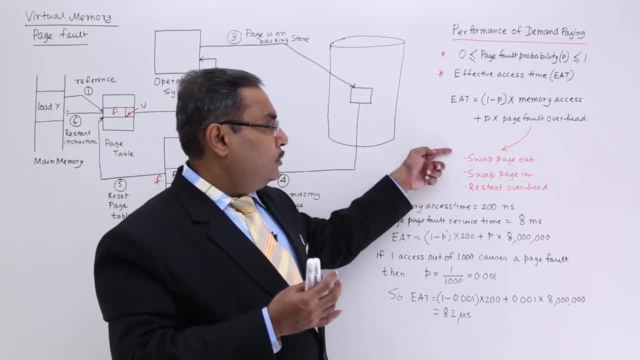 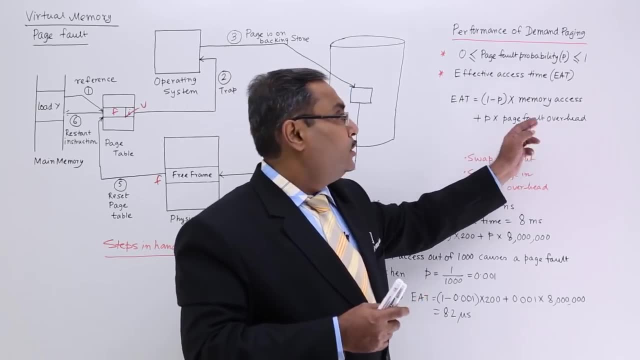 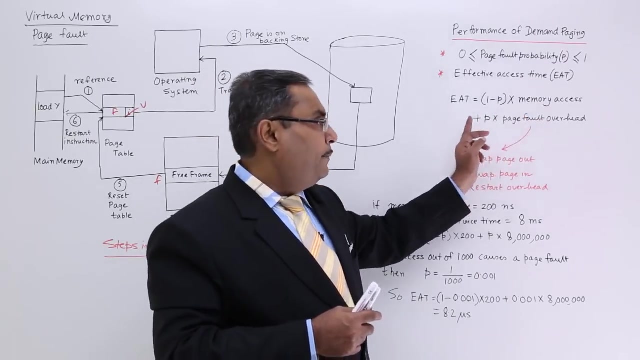 my desired target page is now in the memory. So if you consider all these three time components in total, I shall tell it as page fault overhead. So 1 minus P means occurrence of no page fault. probability of occurrence of no page fault into memory. access time plus probability. 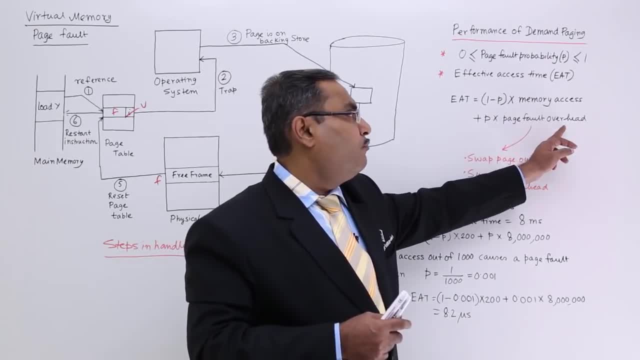 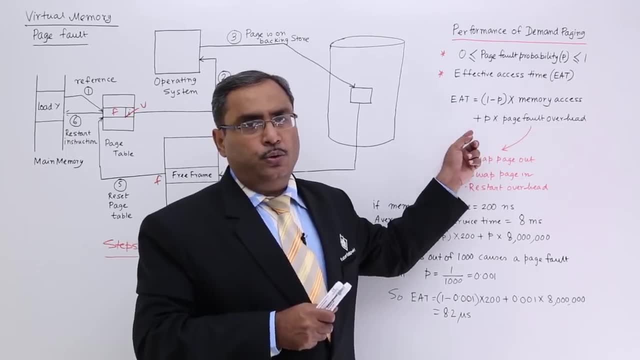 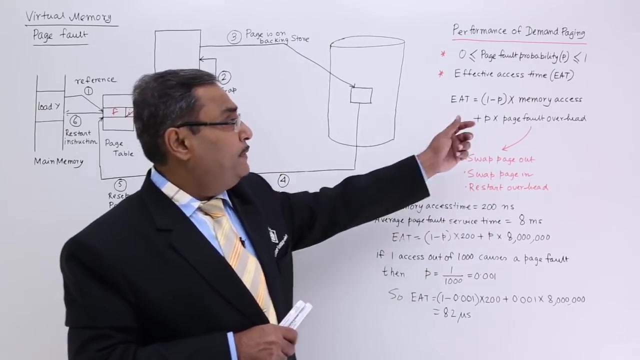 of occurrence of page fault into page fault overhead. So in this way I am going to get a value that is the effective access time. If this conception is not clear to you, let me discuss one numerical problem. So if the memory access time is 200 nanosecond, that 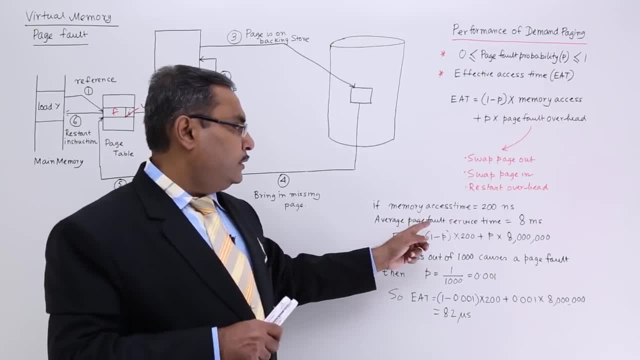 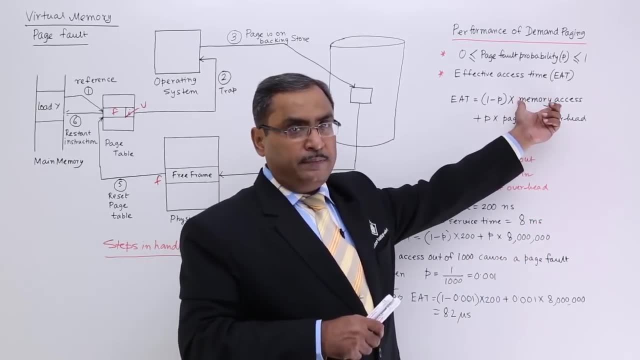 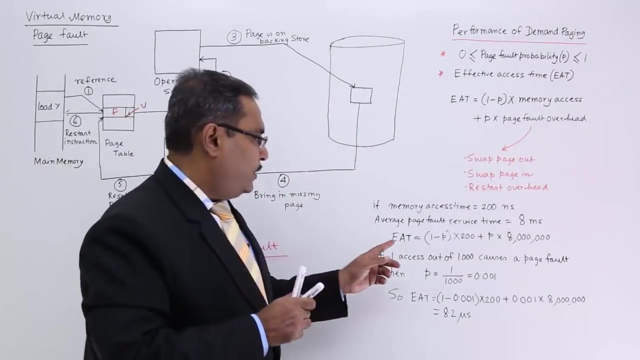 means this value is 200 nanosecond. Page fault service time is 8 milliseconds, So this particular time is 8 milliseconds. So this time is given and this time is given 200 nanosecond and this is my 8 milliseconds. So effective accessing time is equal to 1 minus P into main memory. 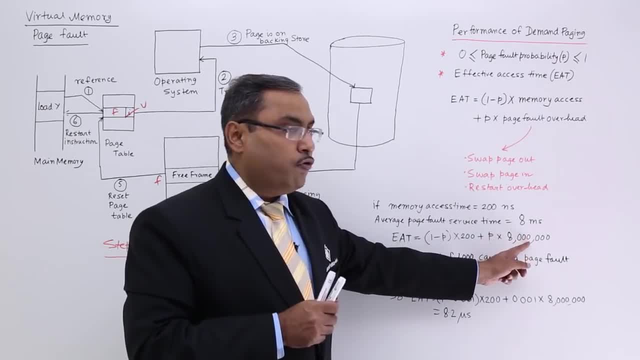 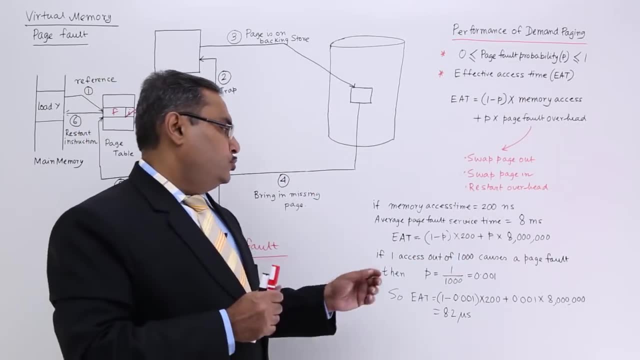 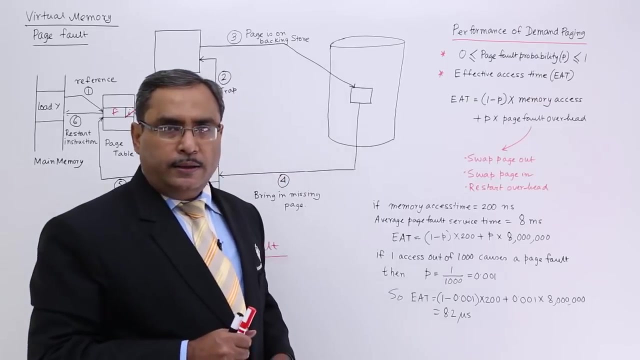 processing time into P, into page fault overhead. So that is the formula. but here P is unknown. until and unless I know P I cannot get the value. So one data is given. if one access out of 1,000 causes a page fault, that means one access out of 1,000 is causing a page. 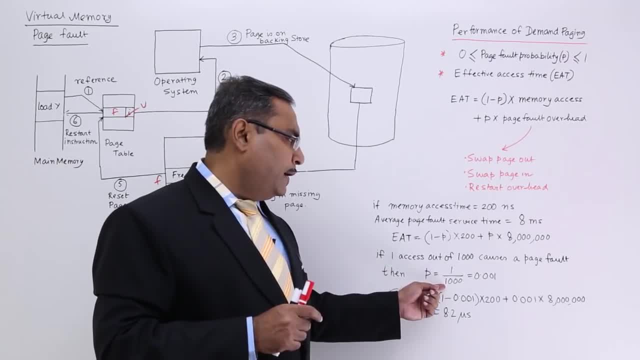 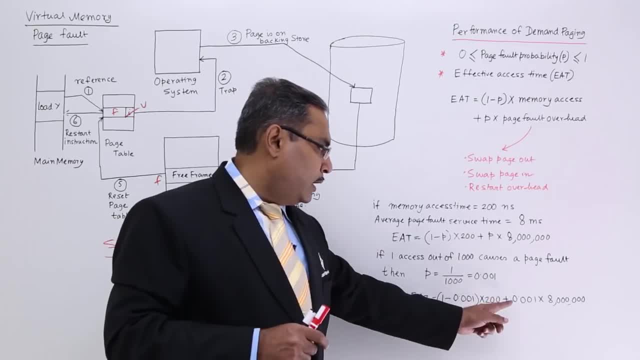 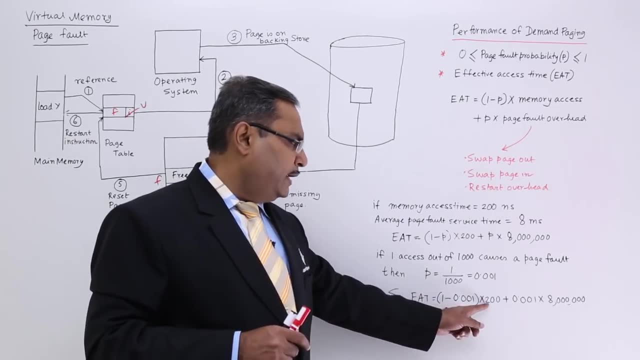 1 minus this and then 0.001 into this. if you put this one So it is, you can easily consider this one as 1.. So it will remain as 200 and here it will become 8000, if you consider this. 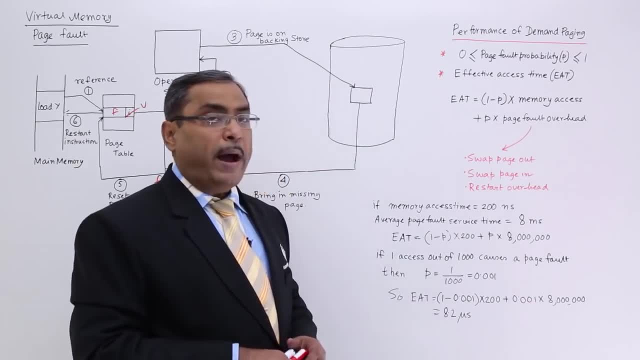 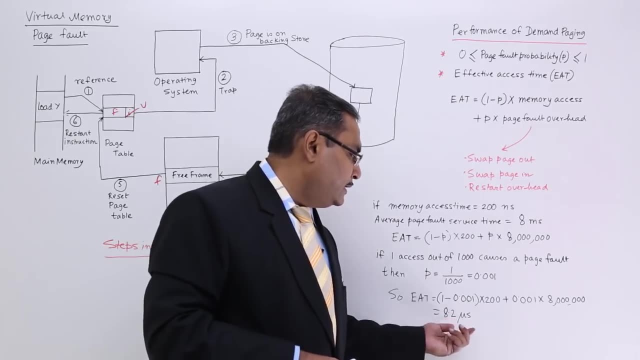 one, 8000.. So it will be 8.2 microsecond. So it have to be 8.2 microsecond. So I am just converting it to the respective same unit, that is, the 8.2 microsecond. So in this, 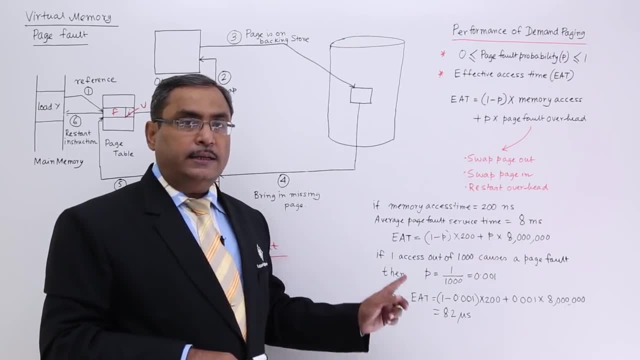 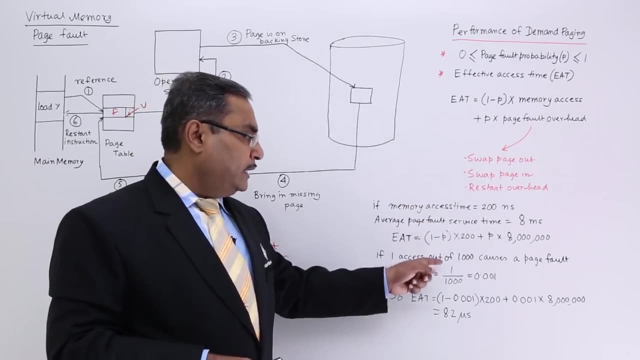 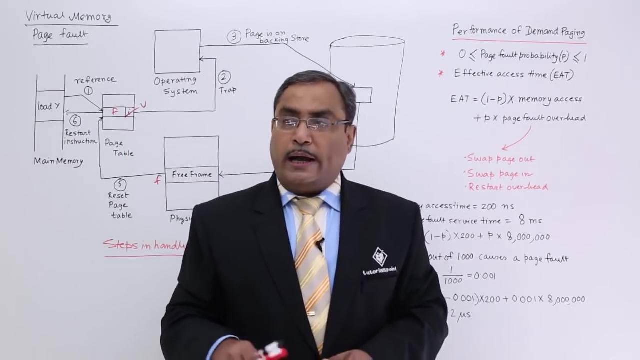 way this sort of problems can be solved in gate exam in the semester exams. such problems are very much probable to come. So please remember this formula and apply this formula. with the given value in the question paper, you will get the effective access time. So 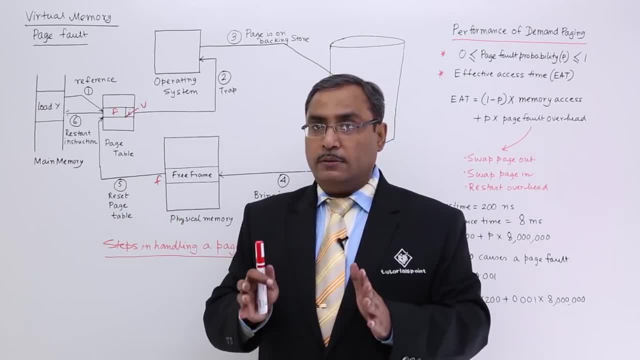 I think you have got this logic how the page fault can be handled by the operating system. Thanks for watching this video. 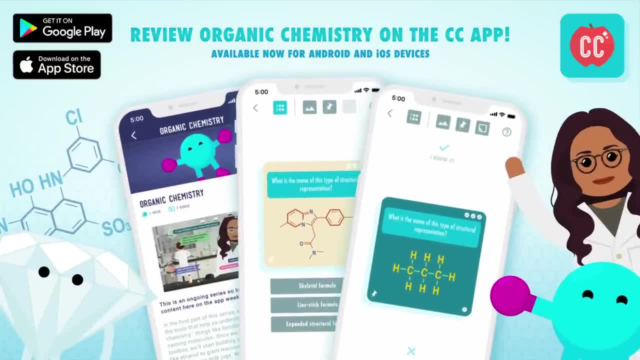 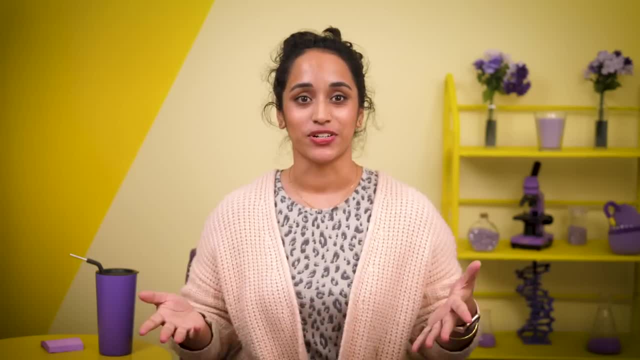 You can review content from Crash Course Organic Chemistry with the Crash Course app, available now for Android and iOS devices. Hi, I'm Deboki Chakravarty, and welcome to Crash Course Organic Chemistry And to my home, where we are filming now Because of the pandemic.